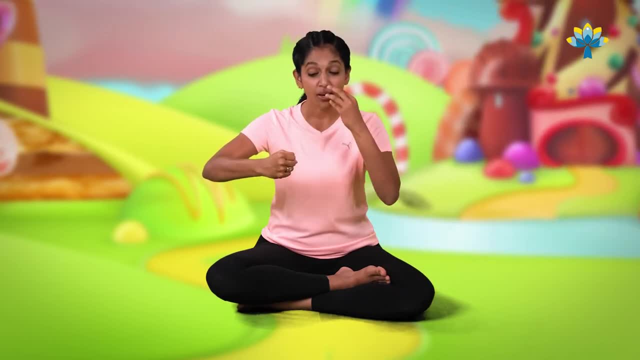 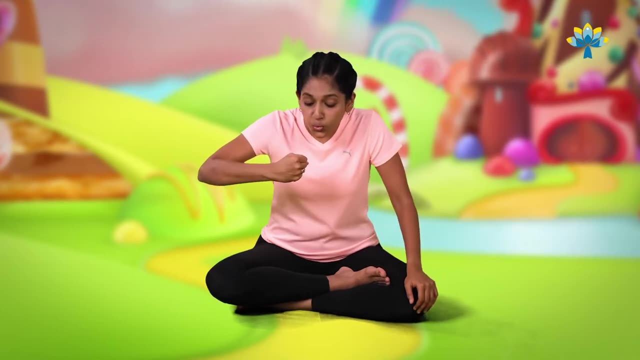 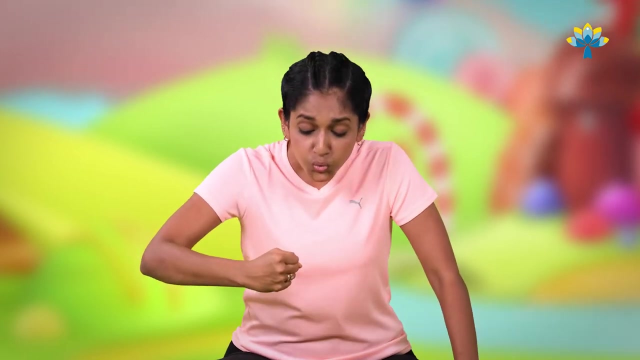 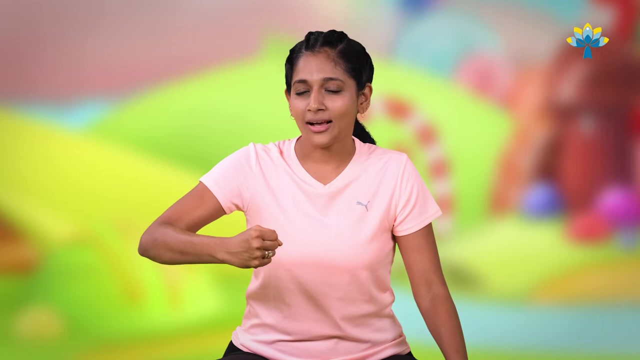 Now. first we are going to strengthen our lungs by blowing air on this hot chocolate so that it can cool down. Let's go Once again One more time. Okay, I think it's a little bit cooler. Now we are going to try to take a sip of this hot chocolate, But when you take a sip, we are going to breathe in through your mouth. 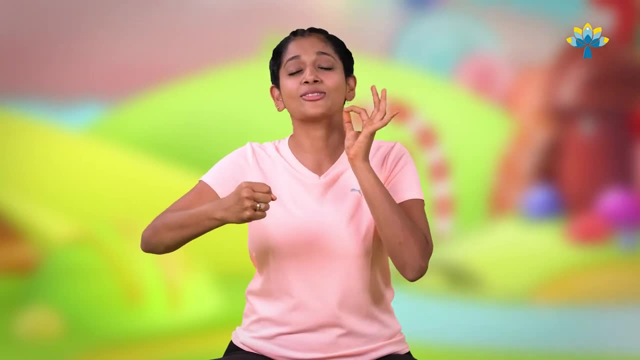 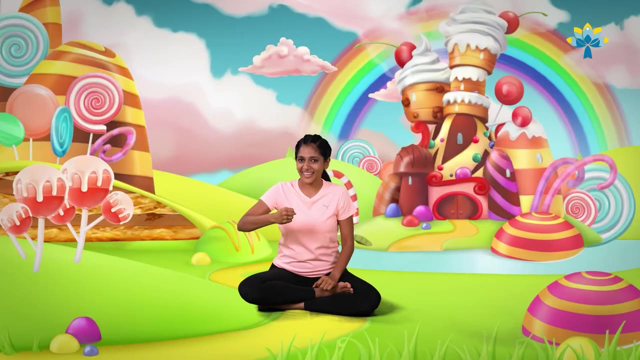 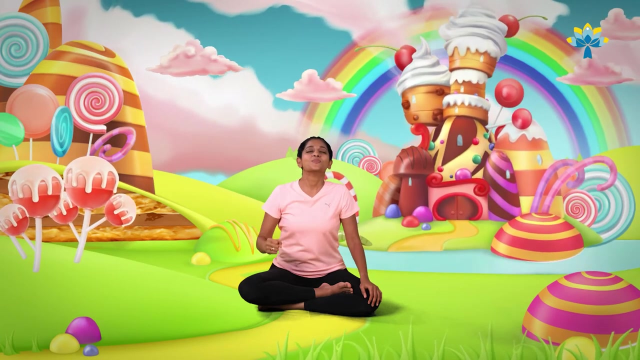 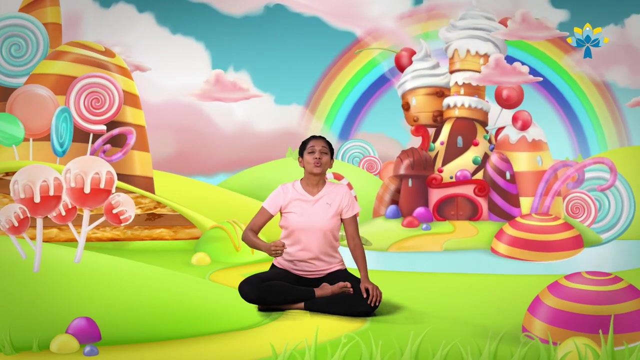 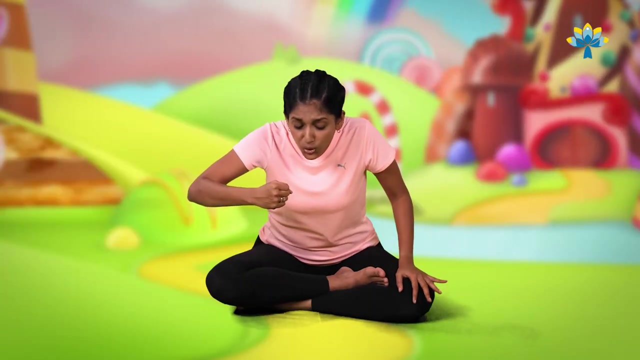 And when you finish drinking that hot chocolate, we are going to say, mmmmm, Okay, Are you ready? Let's take a sip Mmmmm, One more sip Mmmmm. Now let's blow it a little bit more so that it becomes a little bit cooler. 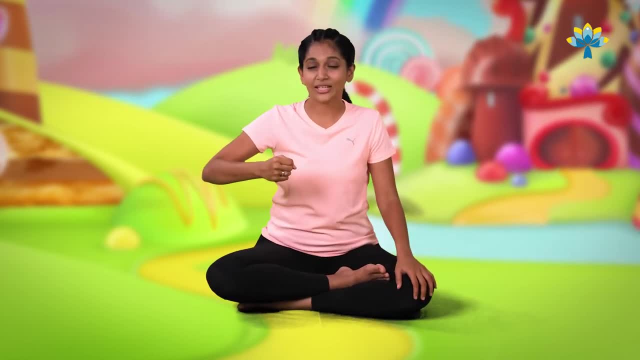 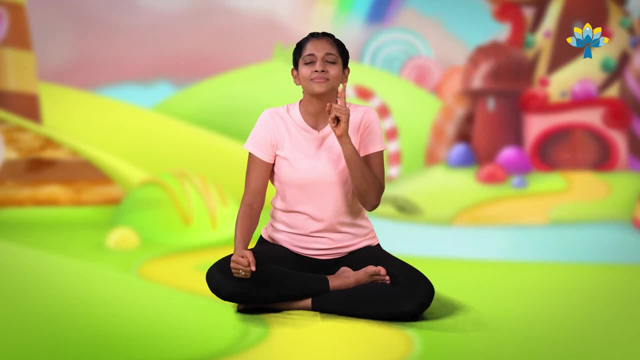 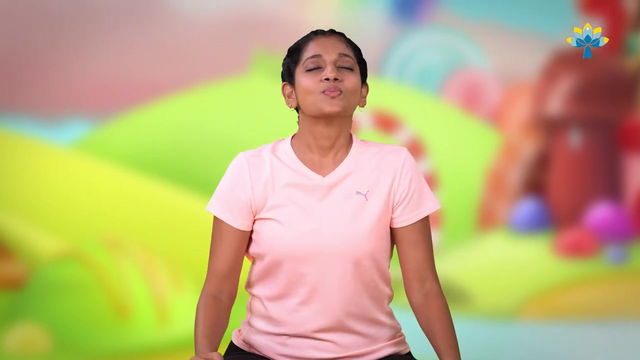 And let's take a few more sips. This time, when you drink this hot chocolate, we are going to go mmmmm, with a little bit more high-pitched tone. Okay, Let's drink that hot chocolate, Mmmmm. 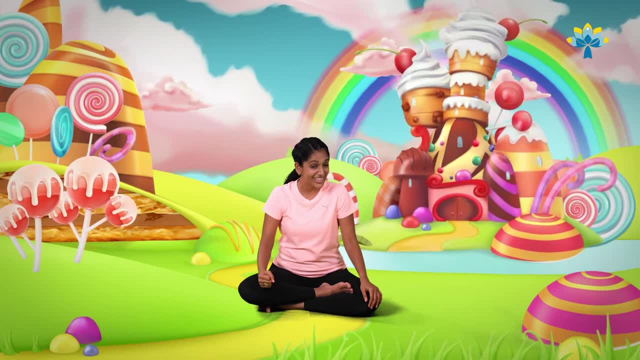 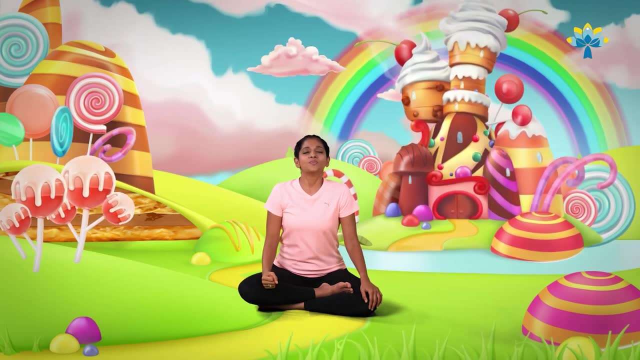 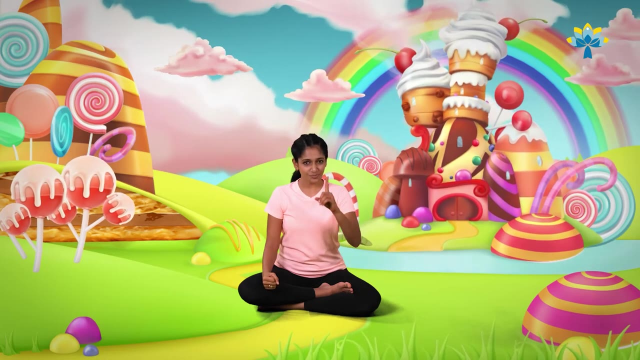 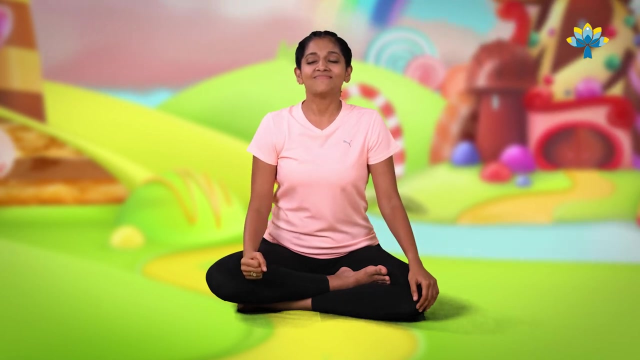 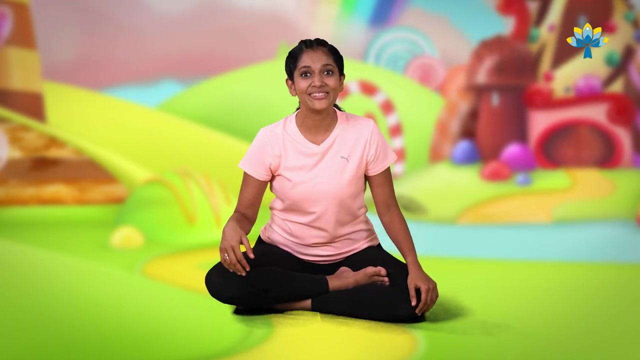 Almost as if this hot chocolate is making you sing. Let's have one more sip, Mmmmm, Mmmmm, Mmmmm, Very good, One last time. Are you ready? Mmmmm, Very nice, Good job. 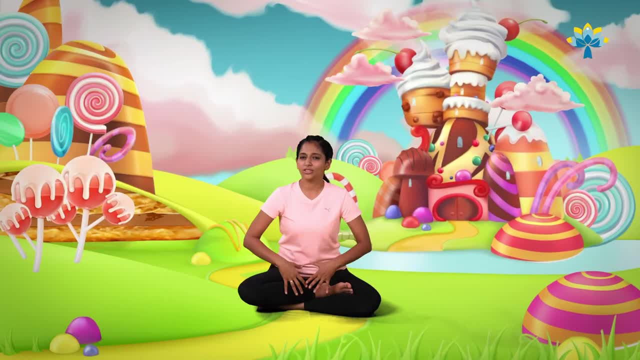 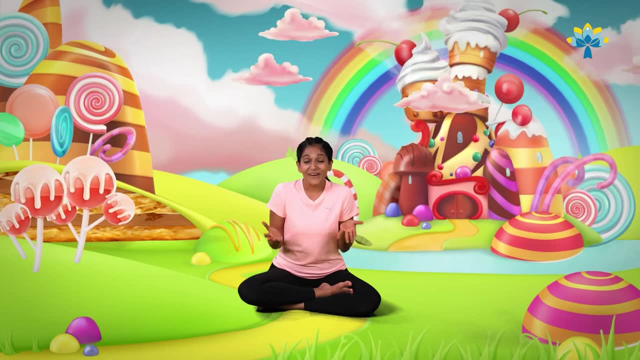 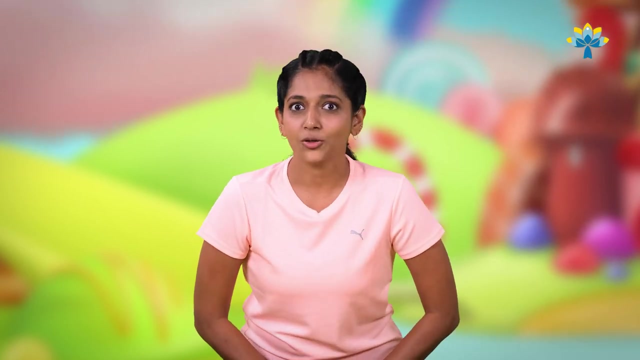 I hope your tummies are feeling full And you are feeling very, very energized To practice lots of yoga with me on our channel, Yoga Gappi. I hope you enjoyed doing the hot chocolate breath and you practice it every single day.